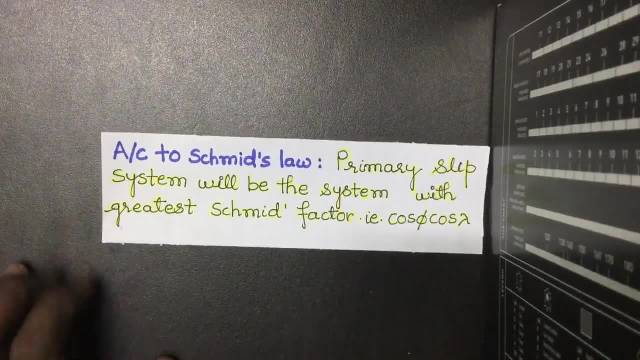 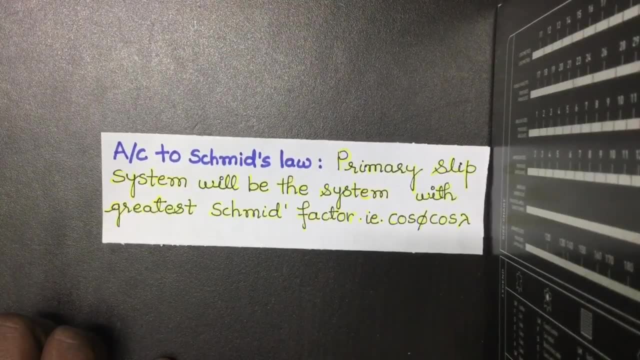 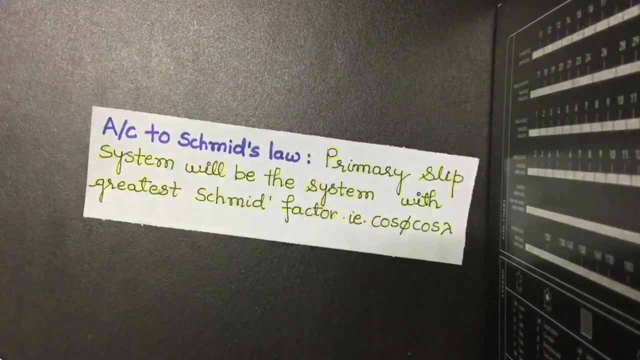 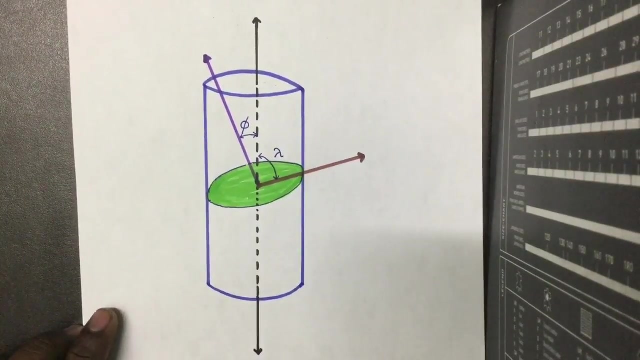 So, and according to Smith law, primary slip system will be the system with the greatest Smith factor. So to solve this problem, you must know about these two concepts. Okay, So first of all I would like to find out the critical resolve, shear stress, The expression for calculation of critical resolve, shear stress. 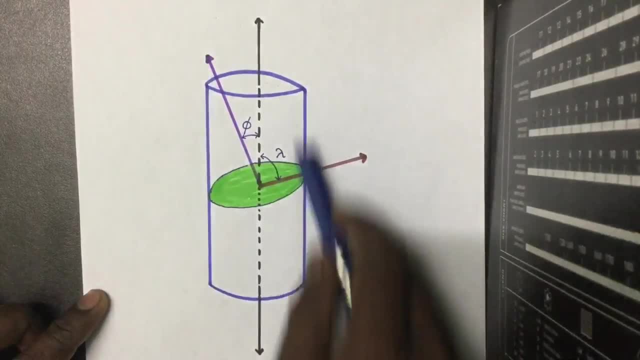 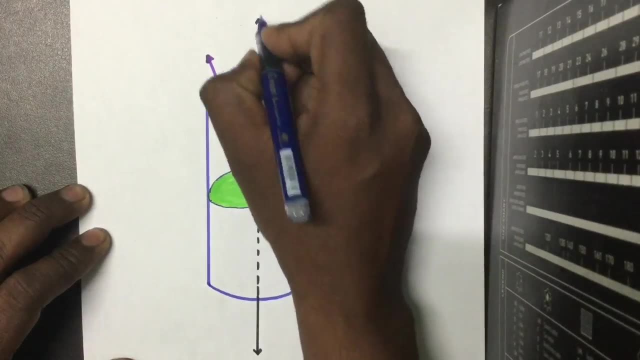 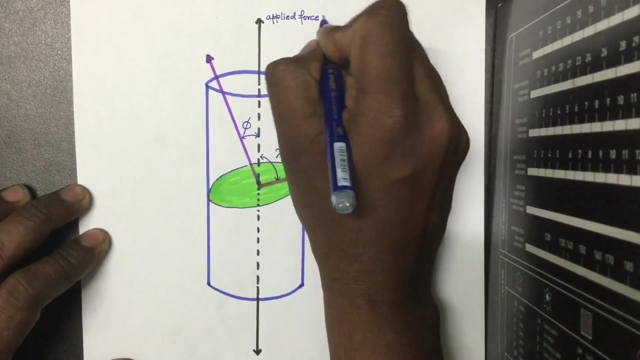 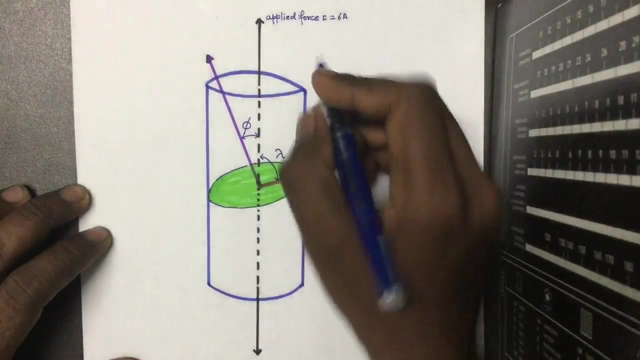 So this is our specimen. You can see, this is our specimen, cylindrical, and this is the direction of applied force. So here, this is the applied force, that is F, and force will be equal to sigma. into a, that is the stress, into, this is the cross sectional area a of this specimen. Okay, 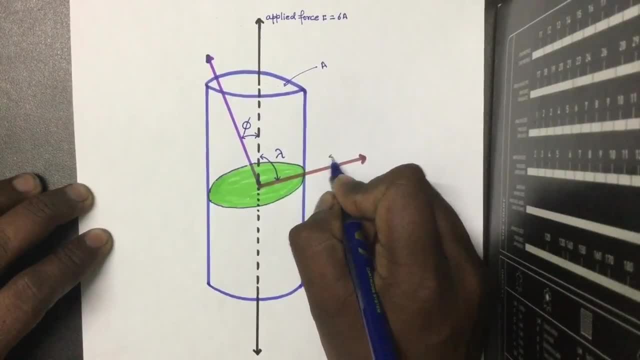 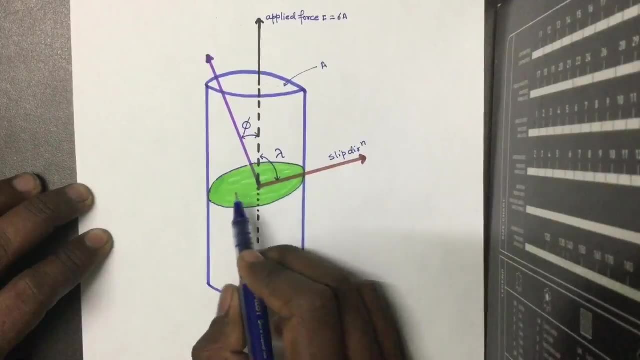 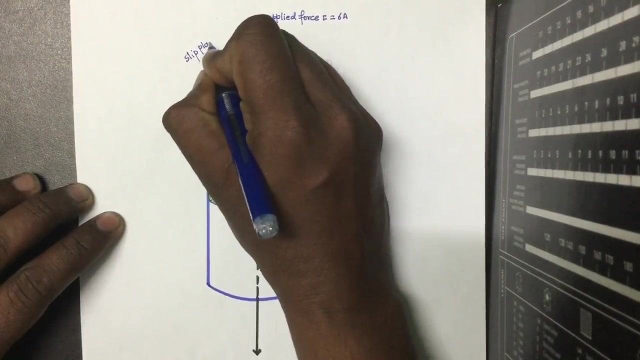 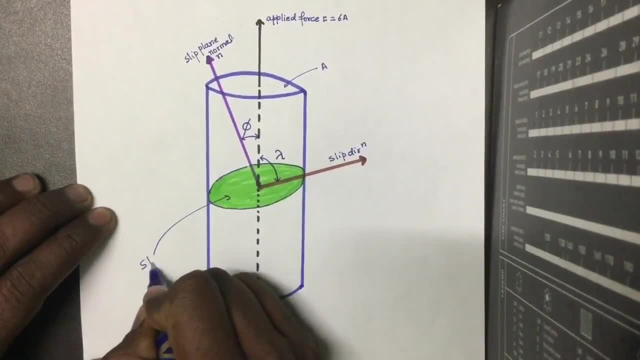 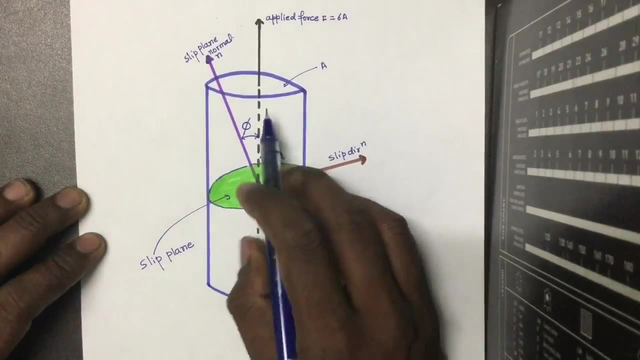 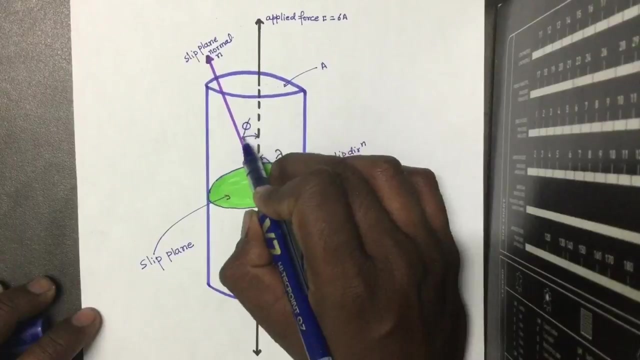 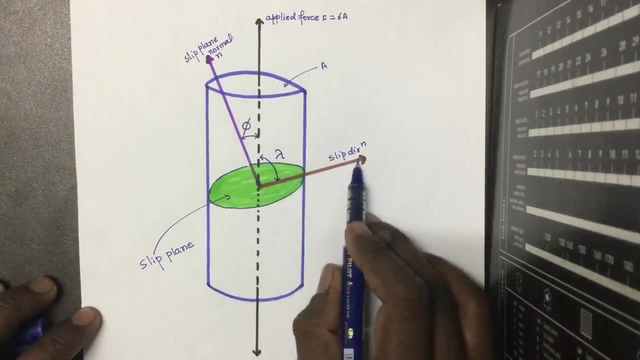 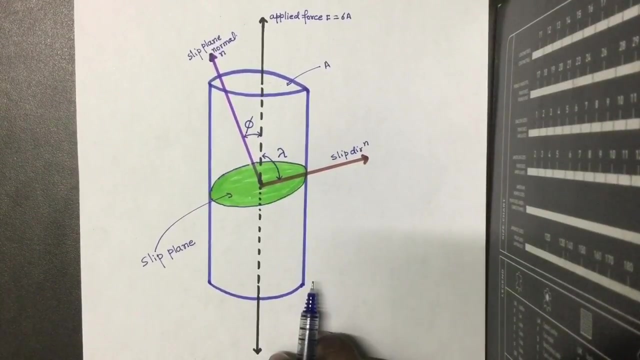 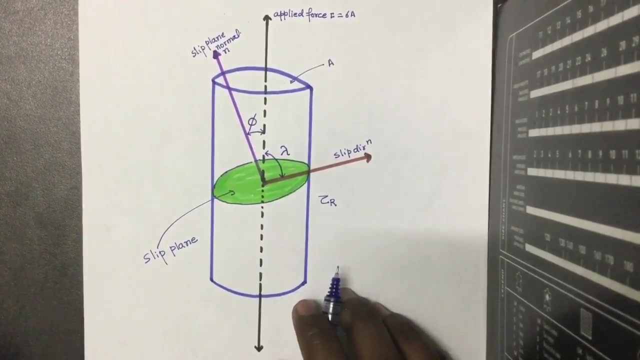 by n and this is our slip plane. This is the angle between the applied force, that is F, and the slip normal, that is phi, and the angle between the applied force and the slip direction is the lambda. So first of all, I would like to find out the tau? r. This is the resolved